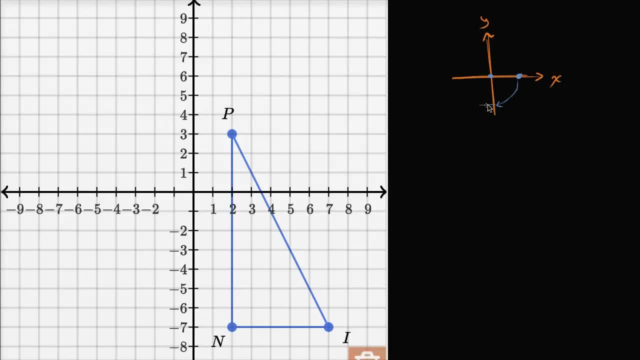 Well, let's see, this would be rotating negative 90. This would be rotating another negative 90,, which together would be negative 180.. And then this would be another negative 90,, which would give you, in total, negative 270 degrees. 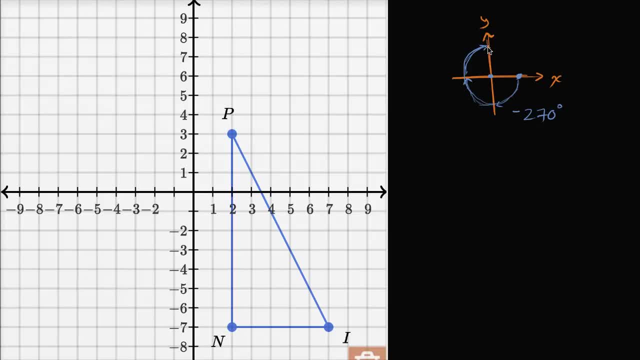 That's negative 270 degrees. Now notice that would get that point here, which we could have also gotten there by just rotating it by positive 90 degrees. We could have just said that this is equivalent to a positive 90 degree rotation. 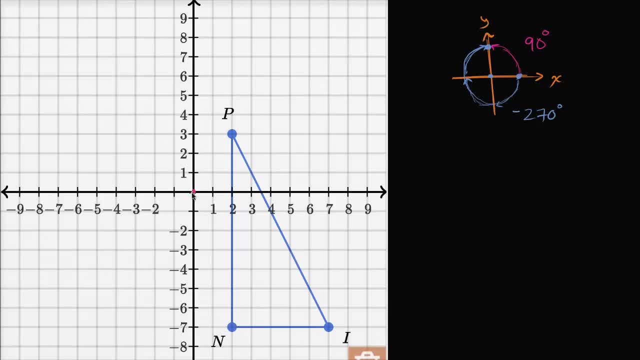 So if they want us to rotate the points here around the origin by negative 270 degrees, that's equivalent to just rotating all of the points, and I'll just focus on the vertices because those are the easiest ones to think about, to visualize. 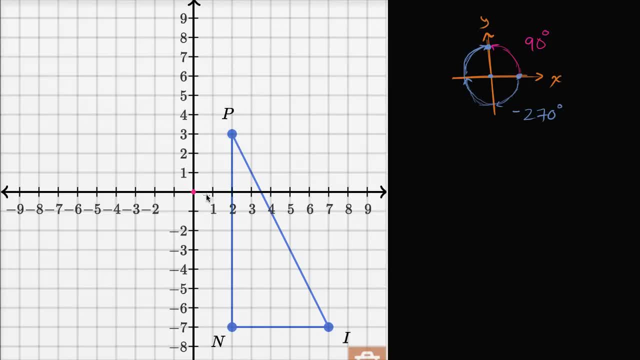 I can just rotate each of those around the origin by positive 90 degrees. But how do we do that? And to do that, what I am going to do to do that, what I'm gonna do is I'm gonna draw a series of right triangles. 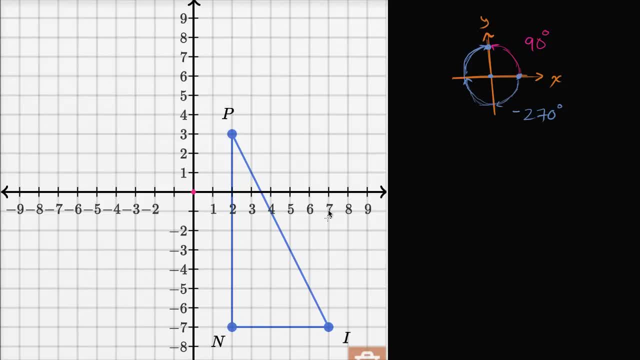 So let's first focus on- actually, let's first focus on- point I right over here and if I were to let me draw a right triangle, and I could draw it several ways, but let me draw it like this, So it's a right triangle. 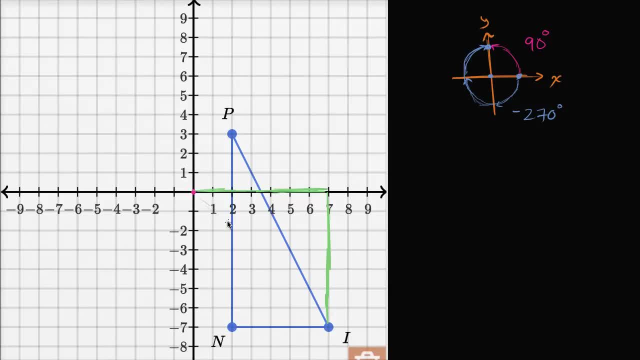 where the line between the origin and I is its hypotenuse. So let me see if I can. it's I could probably draw. I could use a line tool for that, So let me. so that's the hypotenuse of the line. 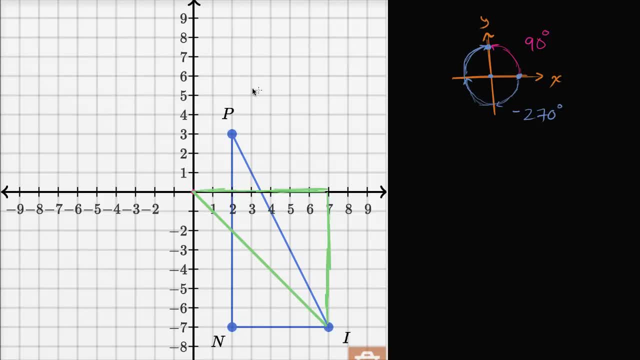 Now, if I'm gonna rotate, I 90 degrees about the origin. that's equivalent to rotating this right triangle 90 degrees. So what's going to happen there? Well, this side right over here, if I rotate, if I rotate this 90 degrees, 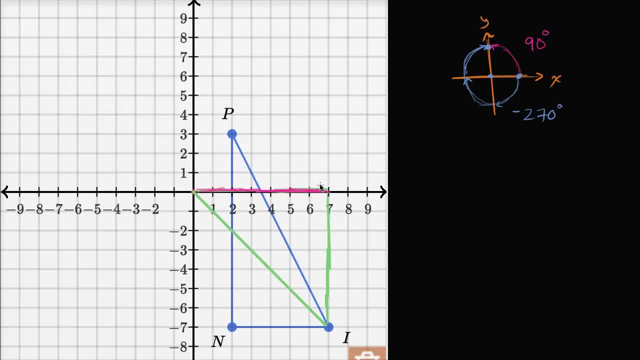 where is that gonna go? Well, instead of going seven along the x-axis, it's gonna go seven along the y-axis. So it's gonna, it's going to. if you rotate it positive 90 degrees, that side is going to look like this: 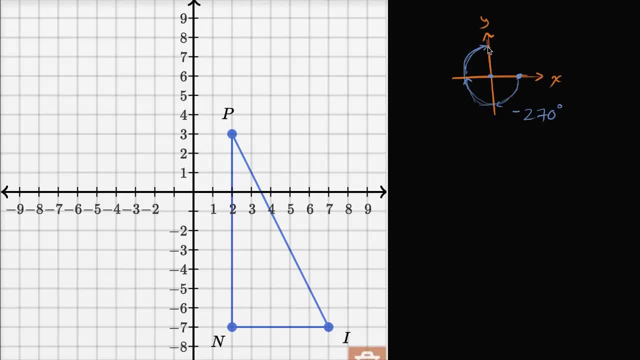 That's negative 270 degrees. Now notice that would get that point here, which we could have also gotten there by just rotating it by positive 90 degrees. We could have just said that this is equivalent to a positive 90 degree rotation. 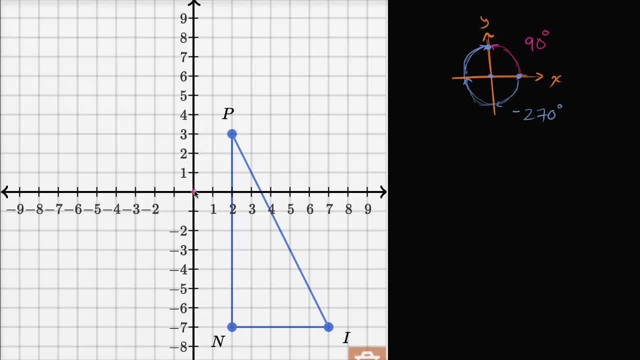 So if they want us to rotate the points here around the origin by negative 270 degrees, that's equivalent to just rotating all of the points, and I'll just focus on the vertices because those are the easiest ones to think about, to visualize. 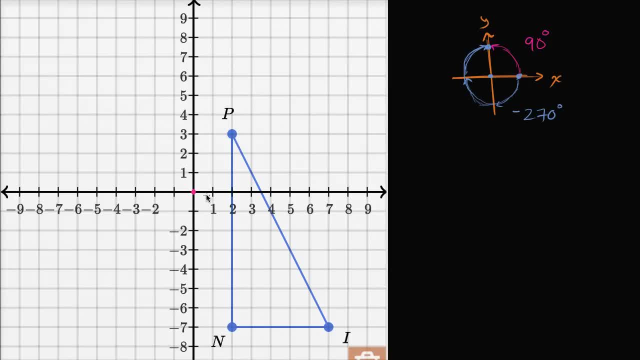 I can just rotate each of those around the origin by positive 90 degrees. But how do we do that? And to do that, what I am going to do to do that, what I'm gonna do is I'm gonna draw a series of right triangles. 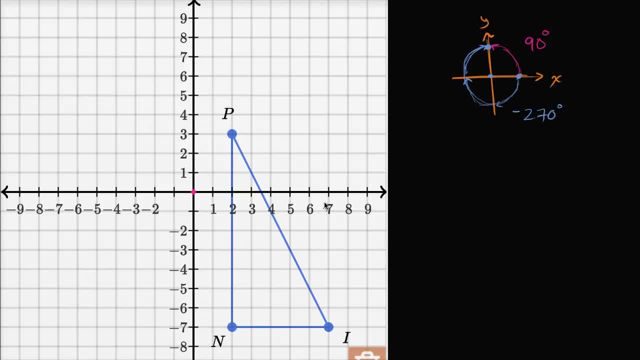 So let's first focus on- actually, let's first focus on- point I right over here and if I were to let me draw a right triangle and I could draw it several ways, but let me draw it, I'm gonna draw it like this: 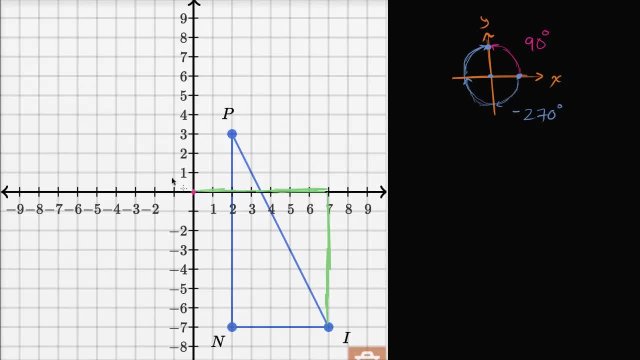 So it's a right triangle where the line between the origin and I is its hypotenuse. So let me see if I can. it's I could probably draw. I could use a line tool for that, So let me. so that's the hypotenuse of the line. 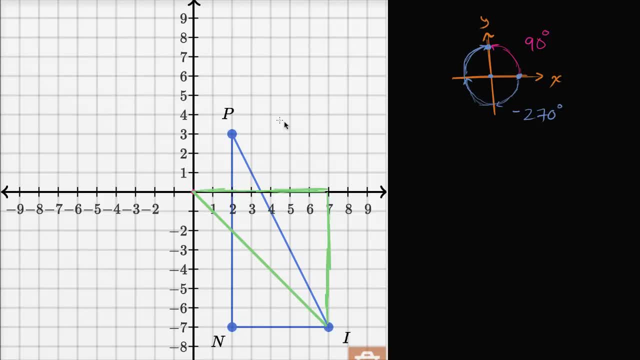 Now, if I'm gonna rotate, I 90 degrees about the origin. that's equivalent to rotating this right triangle. so what's going to happen there? Well, this side, right over here, if I rotate, if I rotate this 90 degrees, 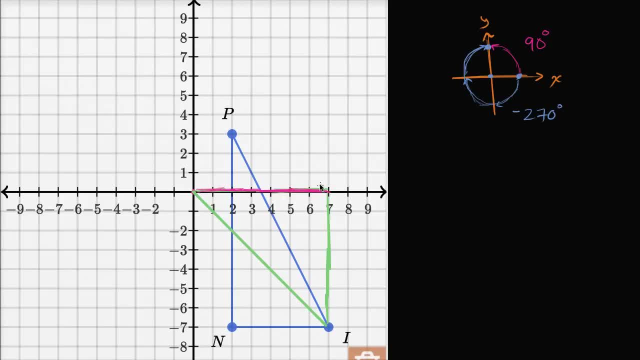 where is that gonna go? Well, instead of going seven along the x-axis, it's gonna go seven along the y-axis. So it's gonna, it's going to. if you rotate it positive 90 degrees, that side is going to look like this: 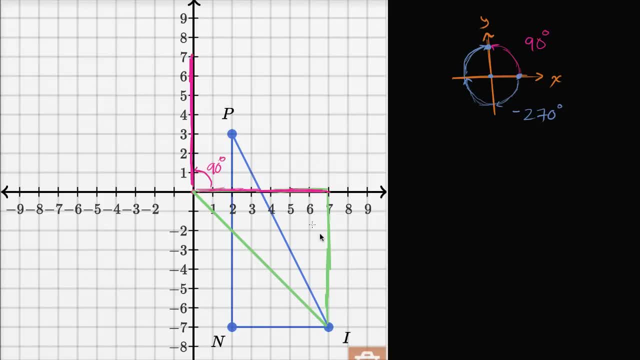 So that's rotating it 90 degrees, just like that. Now, what about this side over here? What about this side? Let me do this in a different color. What about what about this side right over here? Well, this side over here, notice, we've gone down. 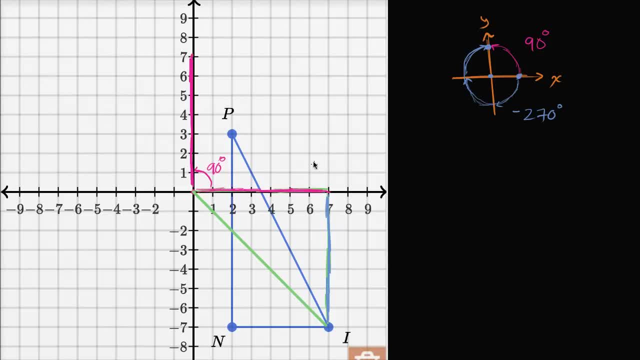 from the origin. we've gone down seven, But if you were to rotate it up, notice this forms a right angle between this magenta side and this blue side. so you're gonna form a right angle again, And so from this point you're gonna go straight. 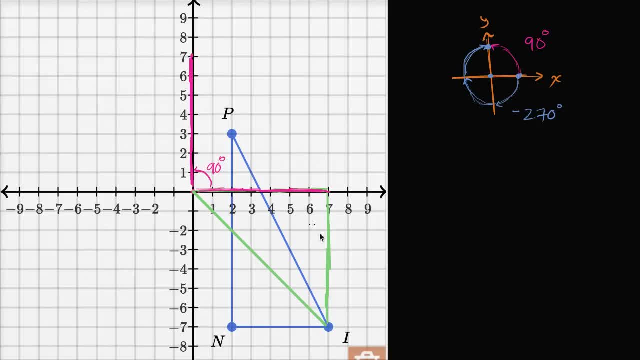 So that's rotating it 90 degrees, just like that. Now, what about this side over here? What about this side? let me do this in a different color. What about, what about this side right over here? Well, this side over here. 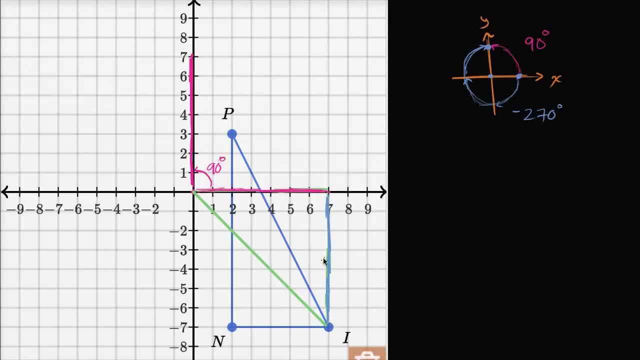 notice, we've gone down from the origin. we've gone down seven. But if you were to rotate it up, notice this forms a right angle between this magenta side and this blue side. So you're gonna form a right angle again. And so, from this point, 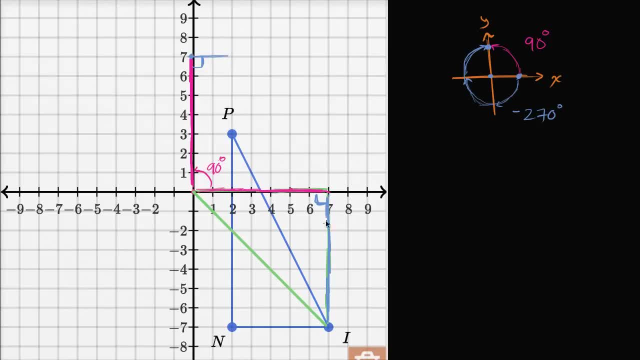 you're gonna go straight as a right angle And instead of going down seven, you're gonna go to the right seven. So you're gonna go. you're gonna go to the right seven, just like this, And so the point I. 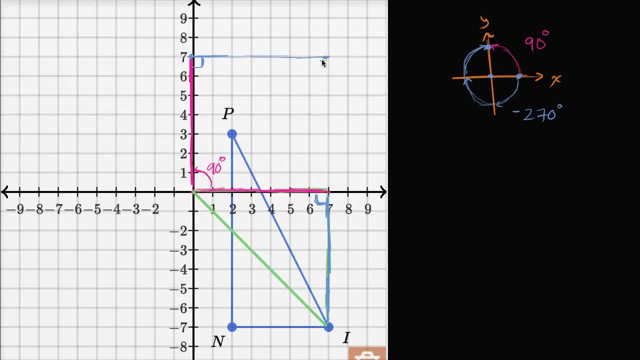 or the corresponding point in the image after. the rotation is going to be right over here. So that green line, let me draw the hypotenuse. now It's gonna look. it's gonna look like whoops. I wanted to do that in a different color. 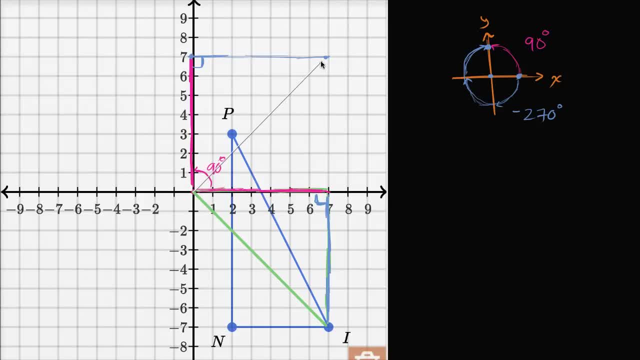 I wanted to do that in the green. I have trouble changing colors. Alright, so there you go, It's gonna look. it's gonna look like that. So your new point: I, if you rotate this triangle, this right triangle, 90 degrees, 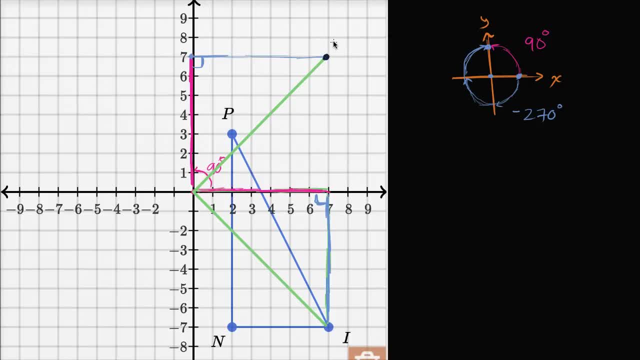 your new point. I maybe I shouldn't say I'll call it I prime, which is what is the image of this point? after I've done, the 90 degree rotation is going to be right over here, And now we can do that for each of the points. 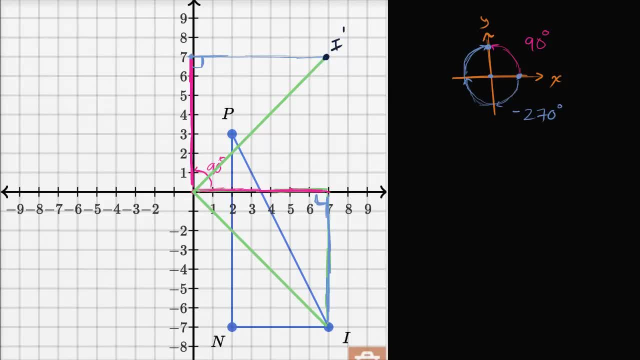 We can do that for N here. Let's draw a right triangle. Let's draw a right triangle, And I could do it a bunch of different ways I could draw it. I could draw a right triangle like this. Let me draw it like this. 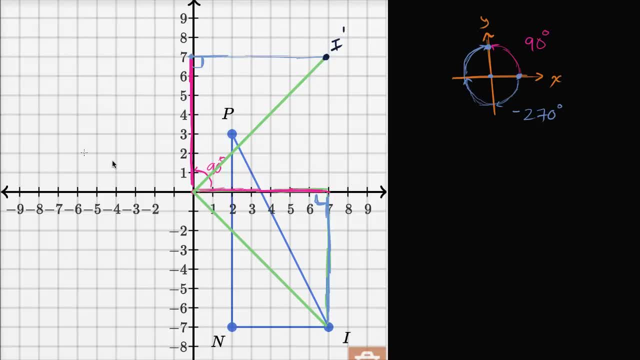 So that's one side of my right triangle. So let me draw the hypotenuse first. So I have the hypotenuse connects the origin to my point, just like that, And then I could- I could either draw it up here. 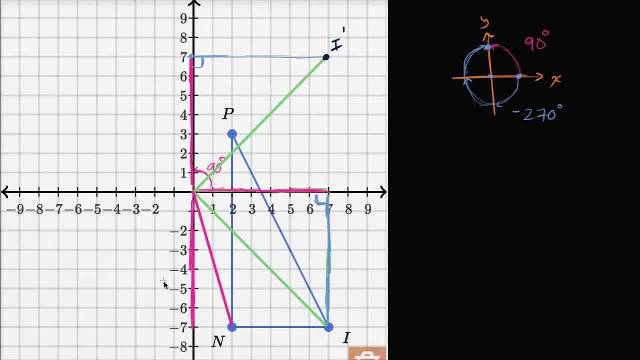 or I could draw it down here like this. I could draw it like this: So if you rotate this 90 degrees, if you rotate this 90 degrees, this side, which is seven units long, and we're going seven below the origin. 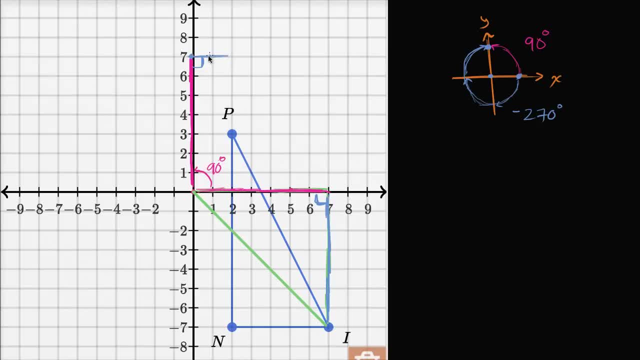 as a right angle, and instead of going down seven, you're gonna go to the right seven. So you're gonna go to the right seven, just like this. And so the point I, or the corresponding point in the image after the rotation: 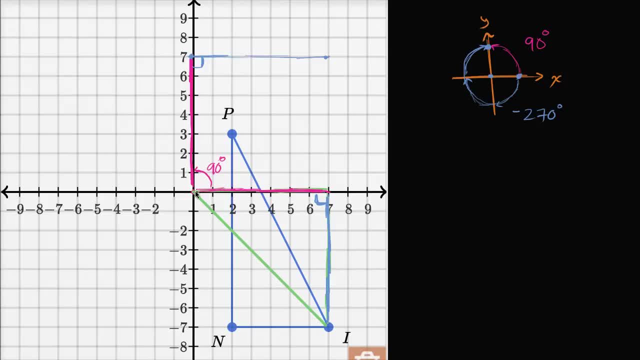 is going to be right over here. So that green line- let me draw the hypotenuse now it's gonna look. it's gonna look like whoops. I wanted to do that in a different color. I wanted to do that in the green. 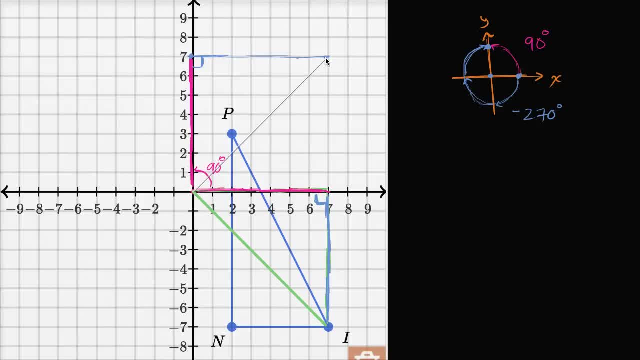 I have trouble changing colors. All right, so there you go, It's gonna look. it's gonna look like that. So your new point I: if you rotate this triangle, this right triangle, 90 degrees, your new point I- or maybe I shouldn't say- 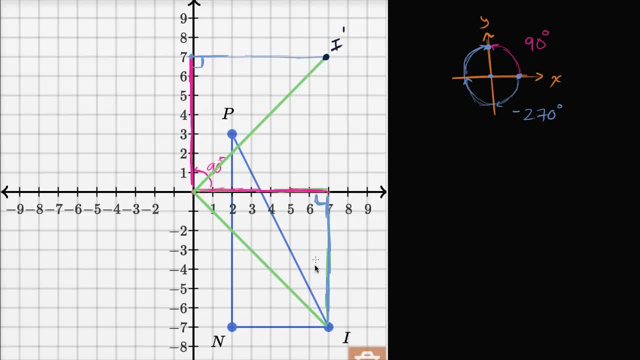 I'll call it I prime, which is what is the image of this point? after I've done, the 90 degree rotation is going to be right over here And now. we can do that for each of the points. We can do that for N here. 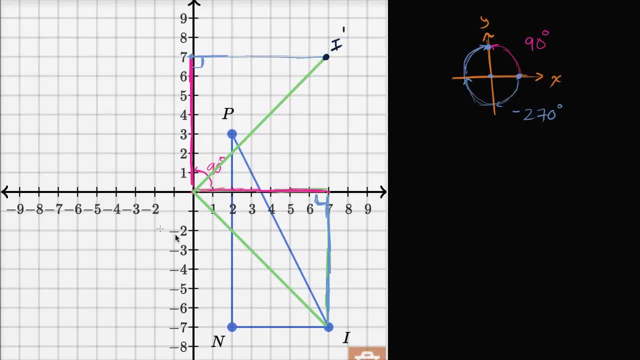 Let's draw a right triangle. Let's draw a right triangle, And I could do it a bunch of different ways I could draw it. I could draw a right triangle like this. Let me draw it like this. So that's one side of my right triangle. 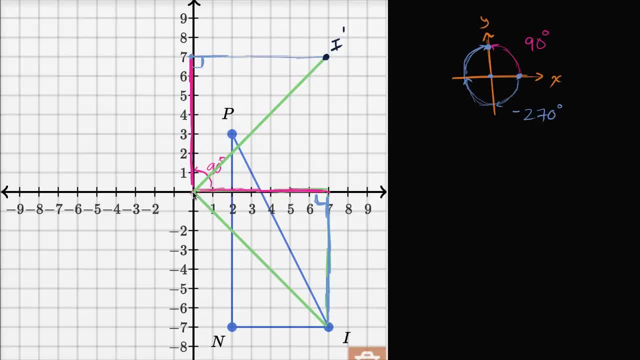 So let me draw the hypotenuse first. So I have, the hypotenuse connects the origin to my point, just like that. And then I could. I could either draw it up here or I could draw it down here, like this: 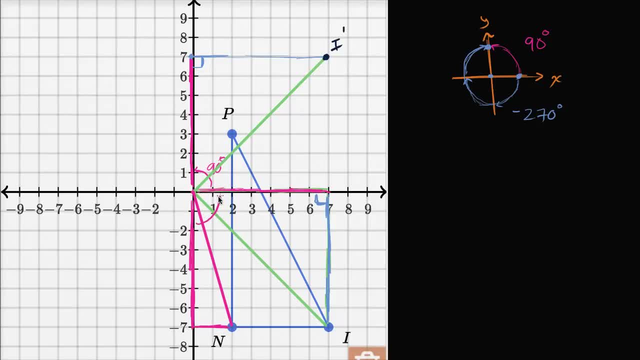 I could draw it like this: So if you rotate this 90 degrees, if you rotate this 90 degrees, this side, which is seven units long and we're going seven below the origin, it's now going to be seven to the right right. 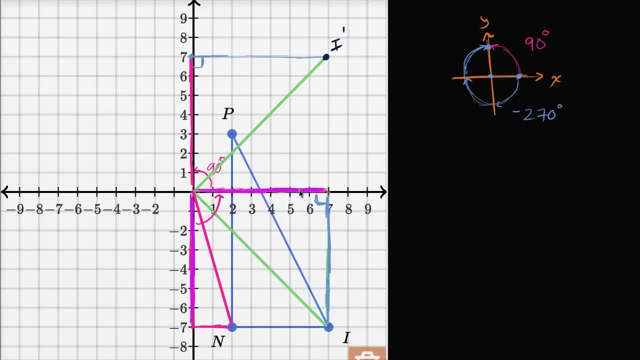 If I rotate it by 90 degrees, it's going to be right over here, It's going to be here. And this side which has length this- let me switch colors- This side which has length two, it forms a right angle. 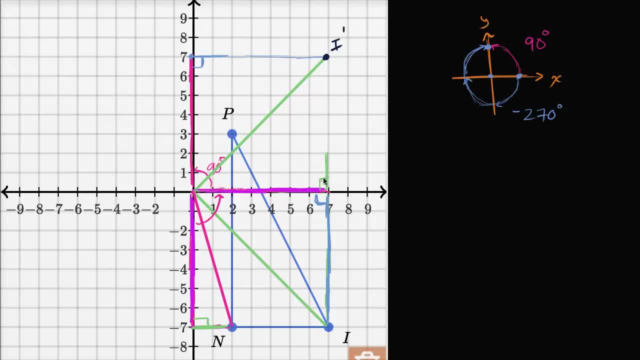 So we're going to form a right angle and have length two right over here, And so your, the image of point N is going to be- let me get the right color, It is going to be just like that. The image of point N is going to be right here. 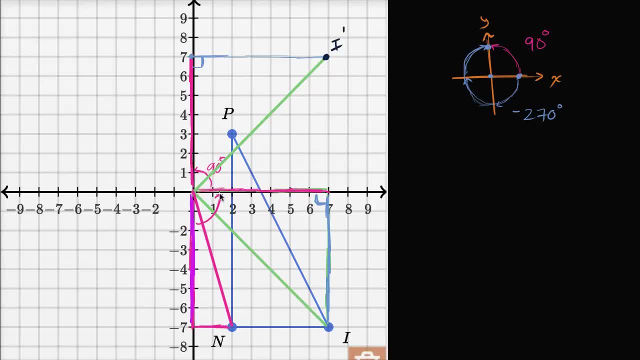 it's now going to be seven to the right. right, If I rotate it by 90 degrees, it's going to be right over here, It's going to be here And this side, which has length this, let me switch colors. 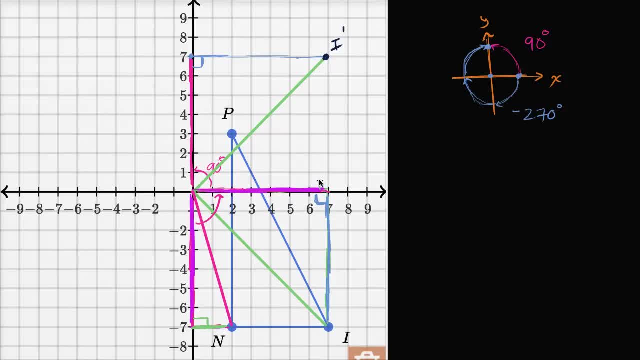 This side, which has length two, it forms a right angle. So we're going to form a right angle and have length two right over here, And so your the image of point N is going to be. let me get the right color. 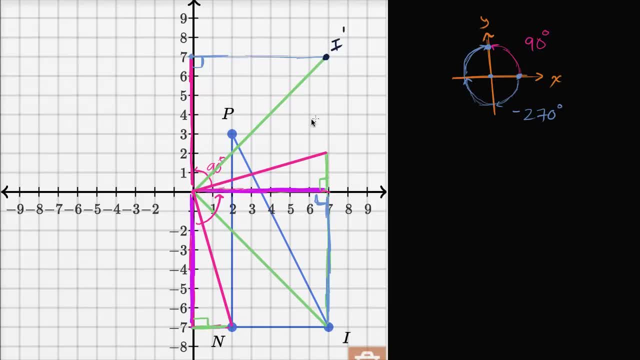 It is going to be like that It is going to be. the image of point N is going to be right here. I'll call that N prime. So we know where the new, where the image of I is the image of N is. 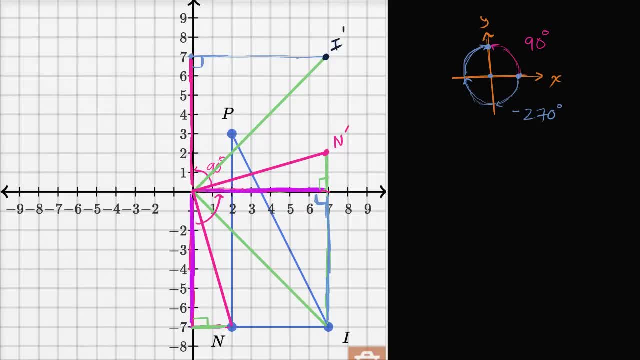 So now we just have to think about where does the image of piece it? And once again we can do our little right triangle idea. So let's draw a right triangle, So just like that I could draw that side And I can do this side right over here. 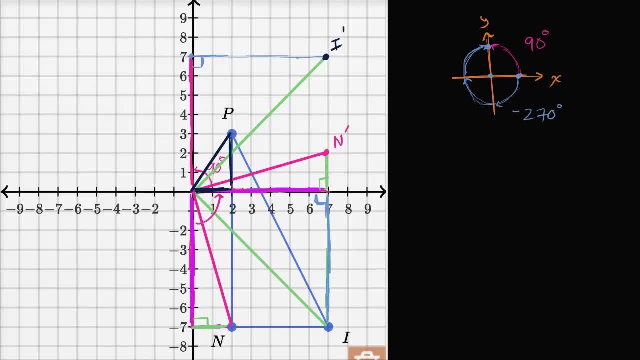 So if I were to rotate, if I were to focus on this, let me do this in a color I haven't. So if I were to focus on, I've already used that color- If I were to focus on this right over here, 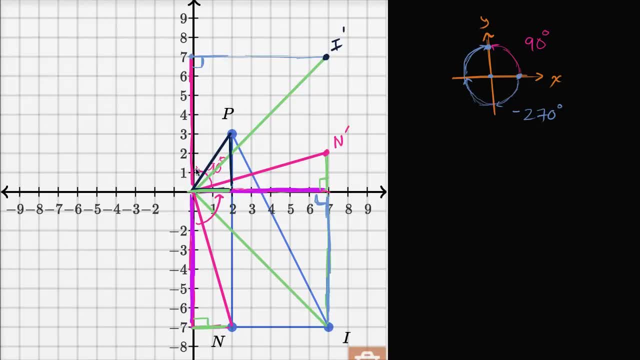 and if I were to rotate it by 90 degrees, instead of going two to the right, it's going to go two straight up. If I rotate this by 90 degrees, it's going to be just like this. Now, this side on. 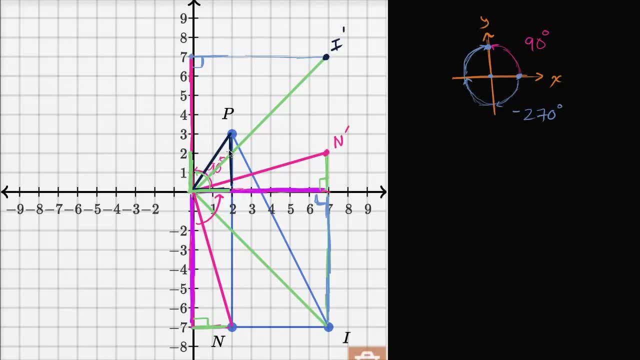 let me pick another color. This side right over here forms a right angle and it has a length of three. So we're going to form a right angle here and have a length of three And just like that we know where the image of P is going to be. 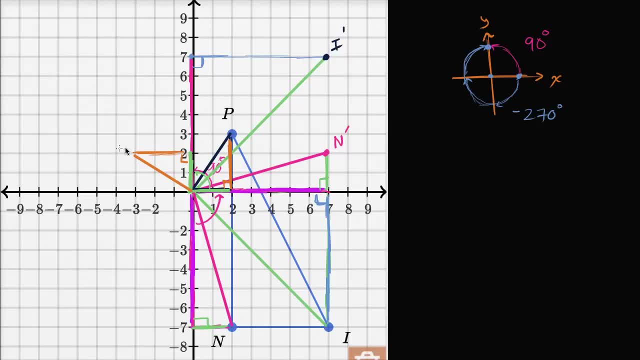 It is going to be. it is going to be right over here. So this is P prime And I know it's kind of confusing, but now we just have to. we now have to connect the P prime, the I prime and the N prime. 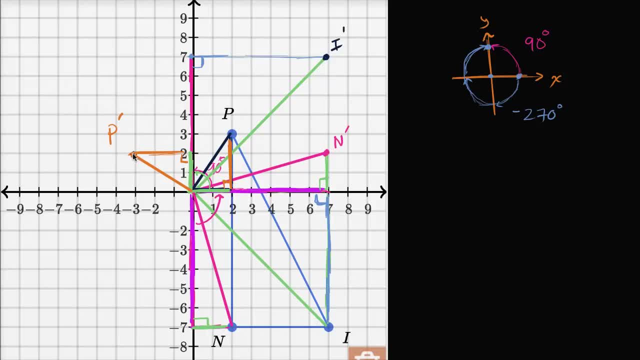 to figure out what the image of my triangle is after rotation. So let me do that. So if I connect these two, I get that. If I connect these two, I get that. And if I connect these two, I connect those two. 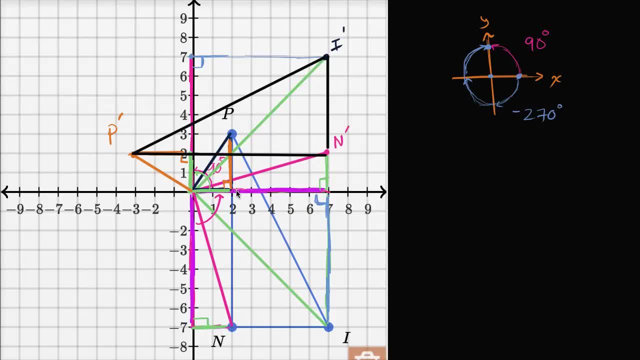 I have that And there you have it. I have the image And now I just have to input it. on the actual problem: So let's see Point negative three comma two, Let me get it out. So negative three comma two is there. 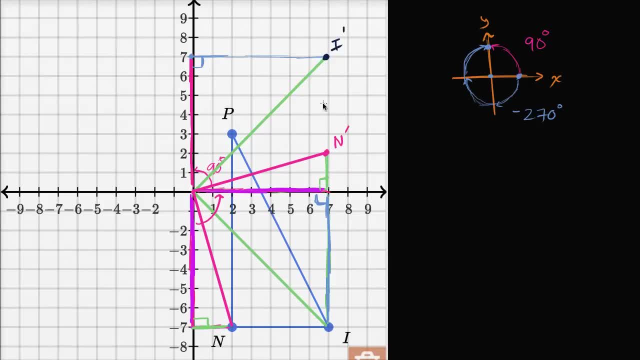 I'll call that N prime. So we know where the new, where the image of I is the image of N, is. So now we just have to think about where does the image of piece it? And once again we can do our little right triangle idea. 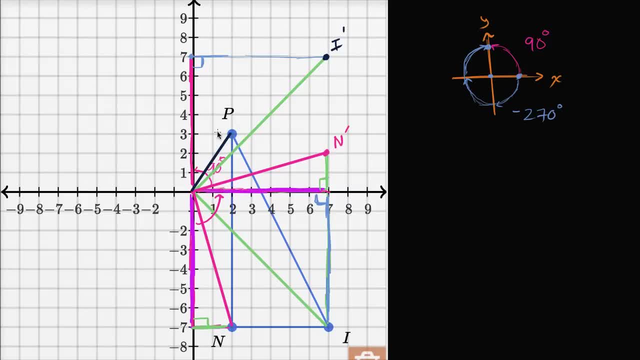 So let's draw a right triangle, So just like that, I can draw that side And I can do this side right over here. So if I were to rotate, if I were to focus on this, let me do this in a color I haven't. 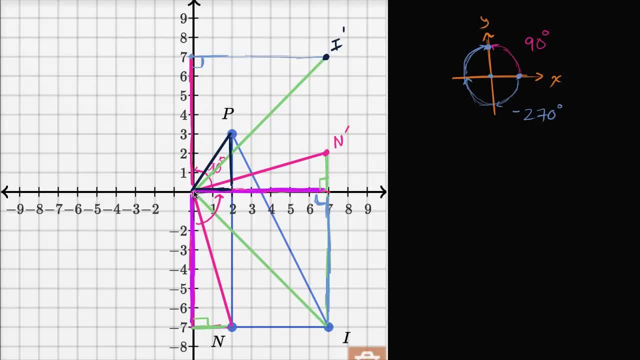 so if I were to focus on- I've already used that color- If I were to focus on this right over here and if I were to rotate it by 90 degrees, instead of going two to the right, it's going to go two straight up. 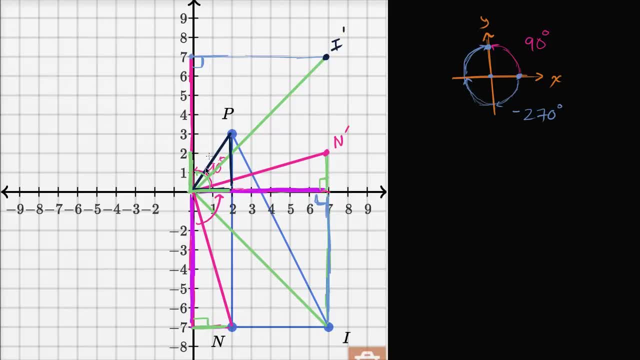 If I rotate this by 90 degrees, it's going to be just like this. Now, this side on- let me pick another color- This side right over here forms a right angle and it has a length of three, So we're going to form a right angle here. 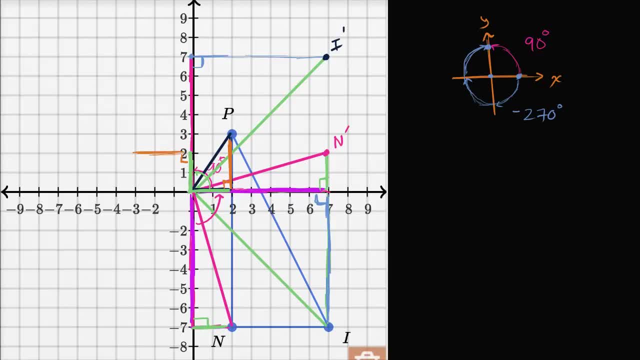 and have a length of three And just like that we know where the image of P is going to be. It is going to be right over here. So this is P prime And I know it's kind of confusing but we now have to connect the P prime. 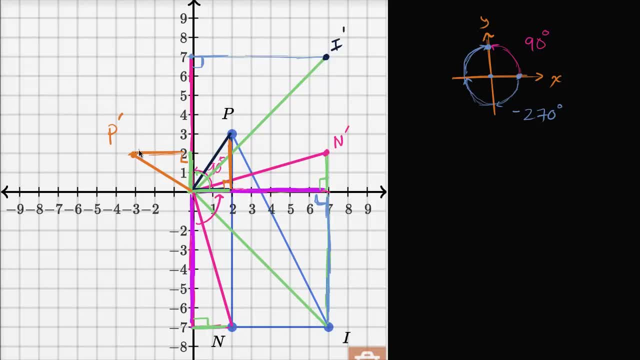 the I prime and the N prime to figure out what the image of my triangle is after rotation. So let me do that. So if I connect these two, I get that. If I connect these two, I get that. And if I connect these two, 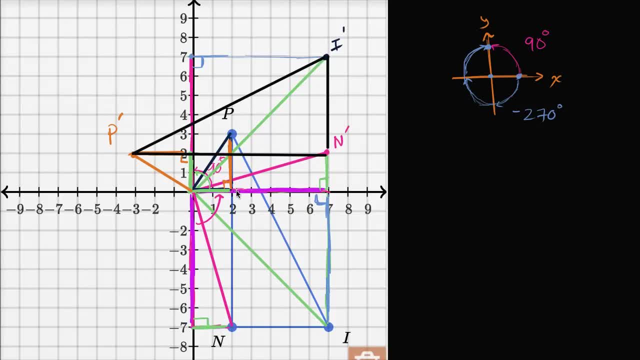 I connect those two. I have that And there you have it. I have the image And now I just have to input it. on the actual problem: So let's see point negative three comma two. Let me get it out. So negative three comma two is there. 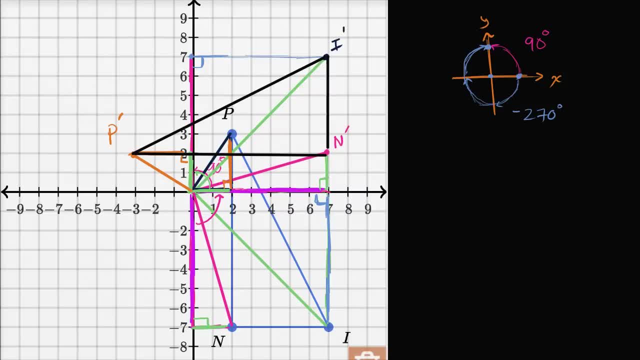 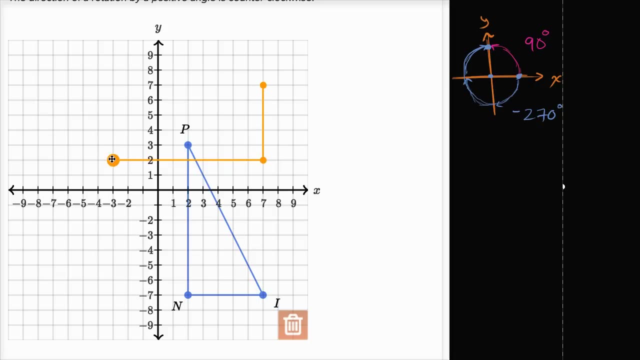 I have seven comma two, So let me put that in there: Seven comma two. And then I have seven comma seven, is there? So let me get this out: So seven comma seven, And then I'll draw it here again to connect the lines. 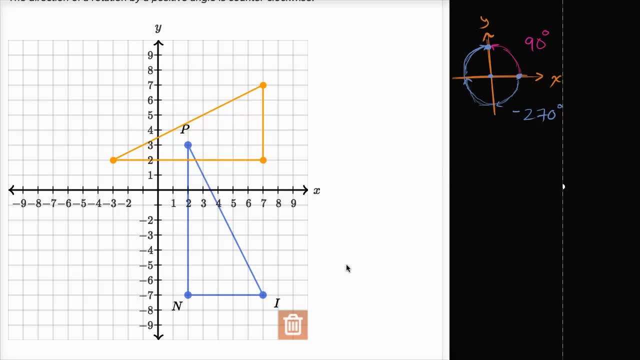 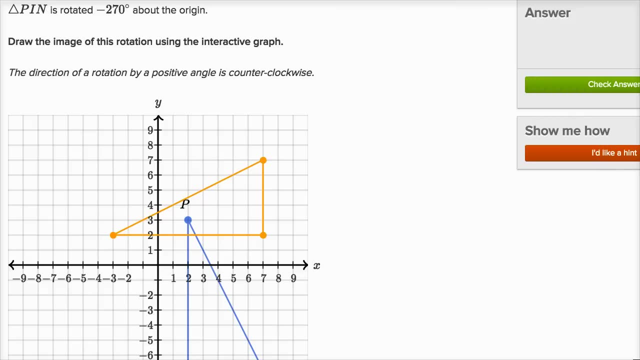 And I'm done. I've rotated it through an angle of 90 degrees, Or negative 270 degrees, which is what they originally asked me for, And I can check to make sure I got the right answer.